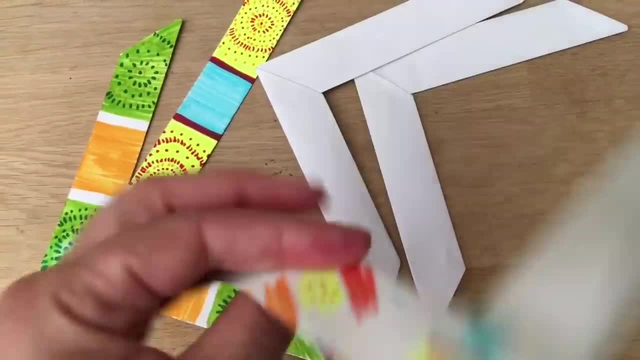 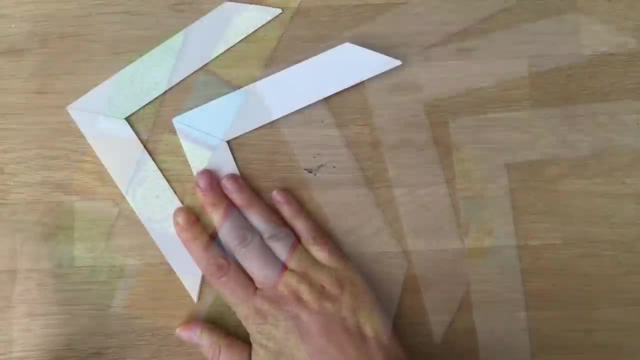 But all you need is a piece of paper, or maybe some old exercise book paper, And if you use printer paper you can obviously decorate them really prettily. So anyway, let's get started and see how to make them. Okay, to make your bookmarks, your boomerangs, you will need a sheet of printer paper. 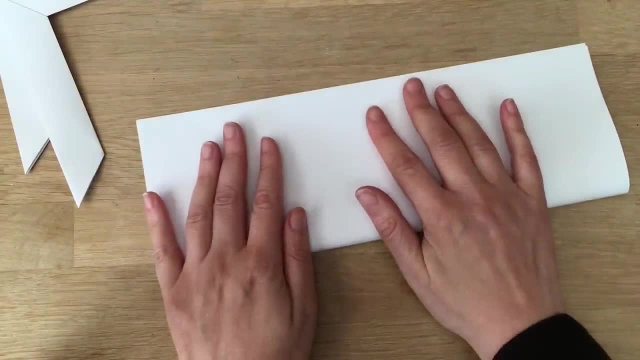 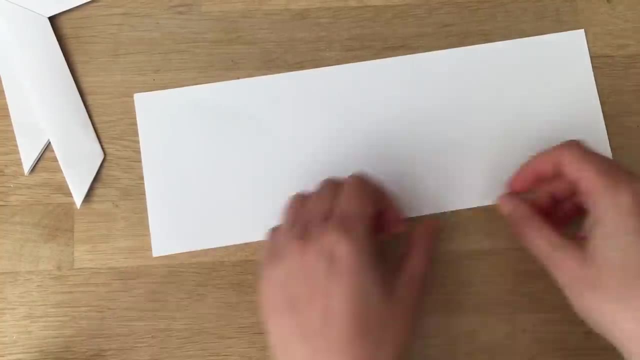 This is the size of a letter paper in the US or A4 here in the UK. Now what you can see me doing here is I'm trying to rip it perfectly in half By doing it, I'm folding it to have all the edges as neat as possible. 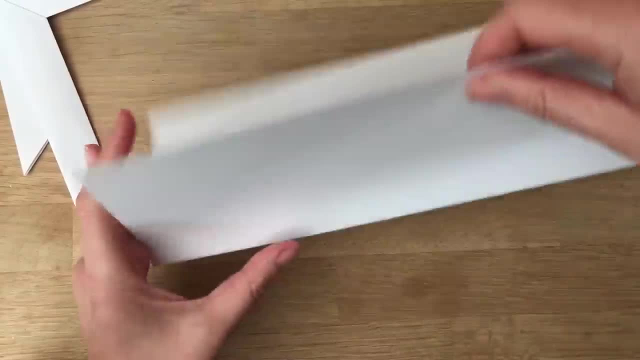 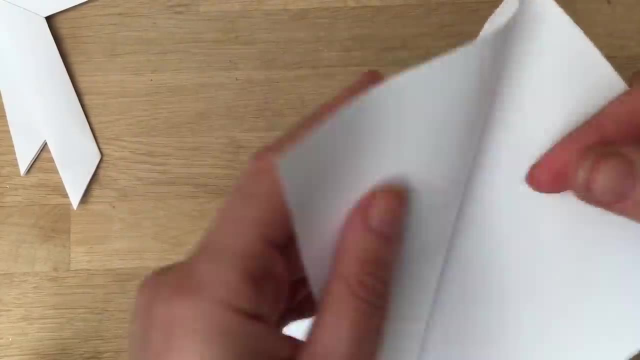 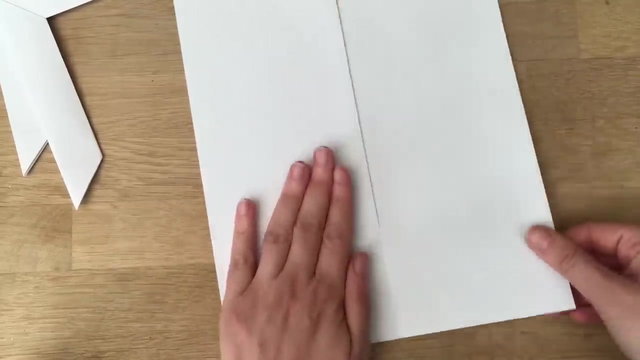 And I'm giving this a super neat line. It's called scoring it, actually, I think so that I can then rip it. So I've scored it and now I'm going to very gently rip it apart. You can, of course, use scissors, but just make sure you cut it. super neat. 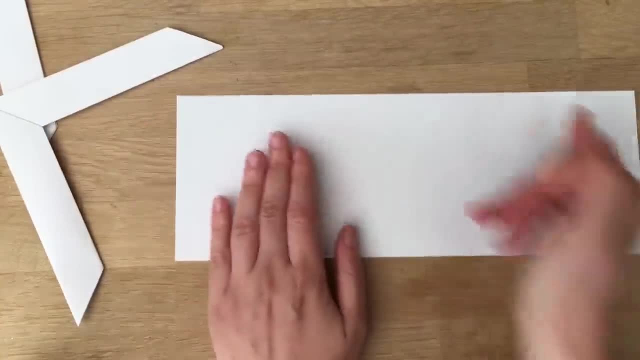 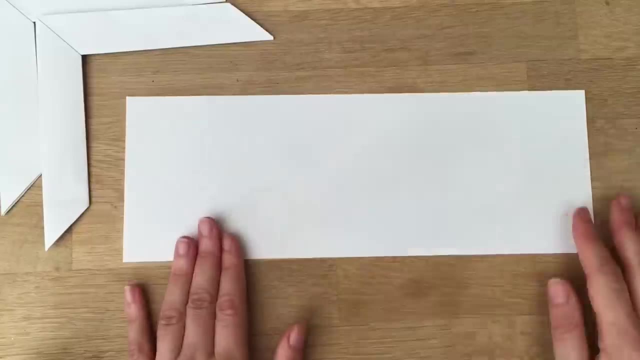 Because it's really important that these are very exact sizes because of the weight and the weight distribution, Because that's how the boomerangs work, So it is important to do this as neatly as possible. So first thing you do is bring this side up and create a fold across the middle. 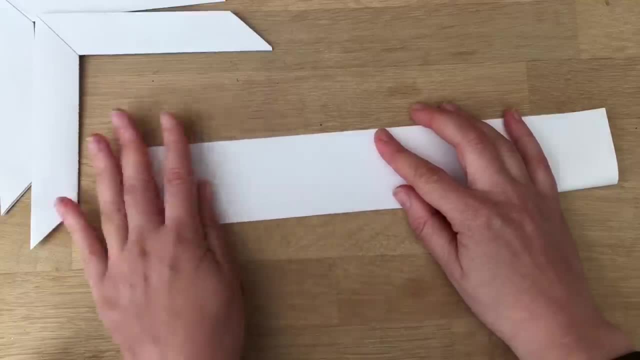 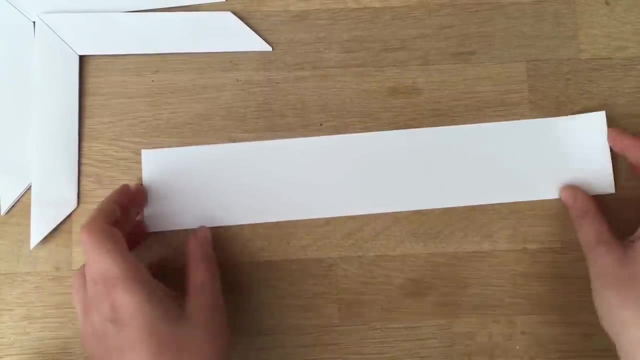 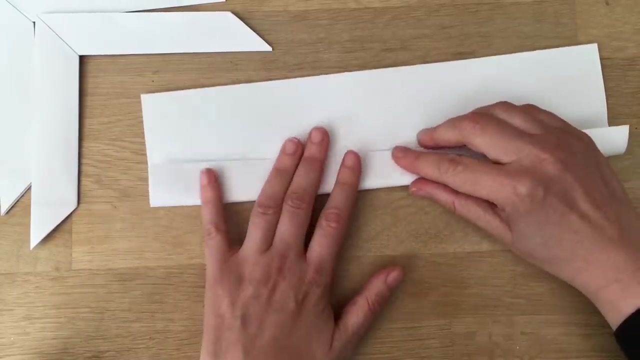 Make sure the edges are aligned on both sides. give it a super neat crease, open it up and now you need to bring the side down and the side up. Now bring them almost to the centre. you don't want them quite to the centre because otherwise things will overlap later. 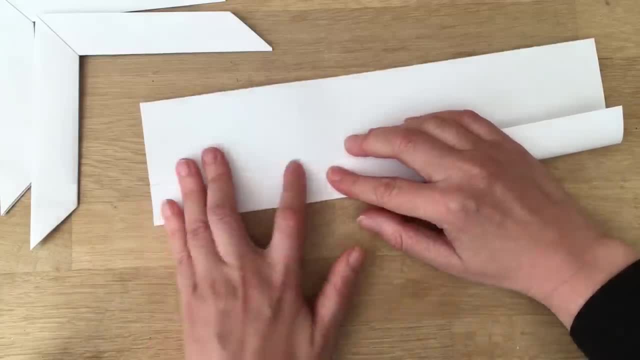 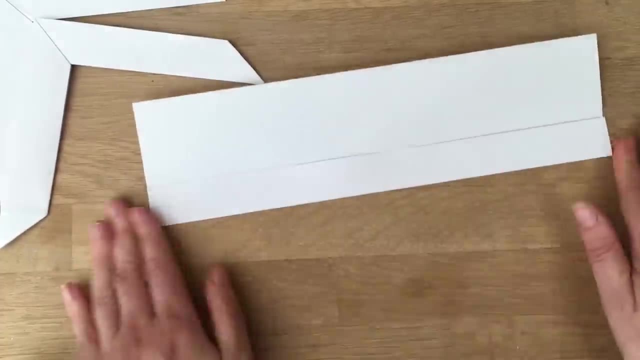 If you do it like a tiny, almost like half a millimetre away, that will allow things to align better. Now make sure the edges are really straight, Really straight, aligned, really neat crease. again, I'm making sure this is very straight and this is very creased. 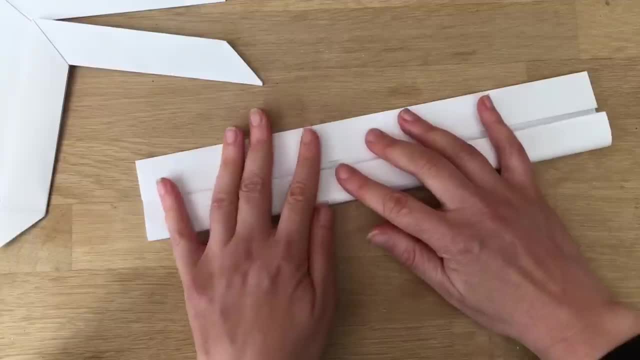 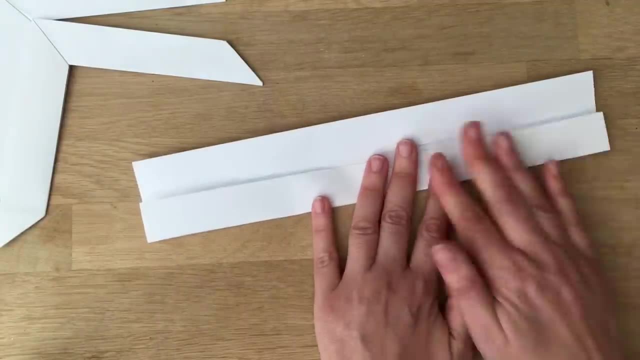 This is probably one of my neatest origamis. Most of the other ones- if you kind of make a little bit of a mistake, it doesn't matter so much, or if you're not 100% neat, But on this one you really do have to work as neatly as possible. 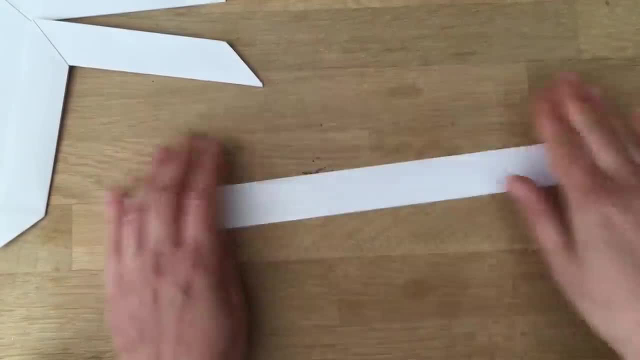 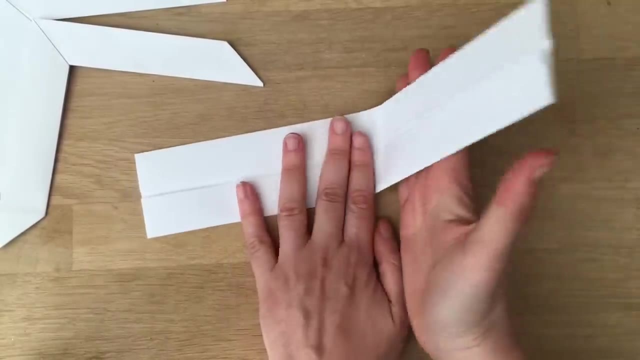 So you can see my lines. don't go all the way to the middle. Here we go. I'm just making sure they're super neat. There we go all and super creased. Now you bring this All the way over, Like so? 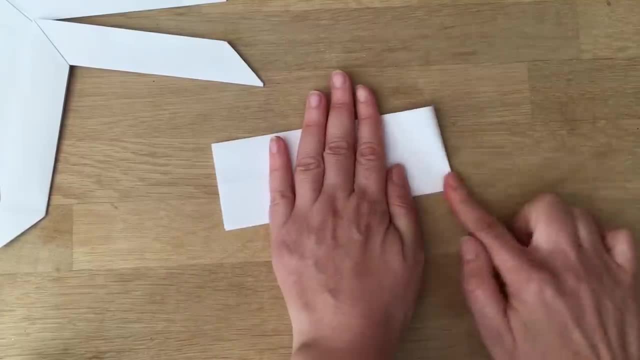 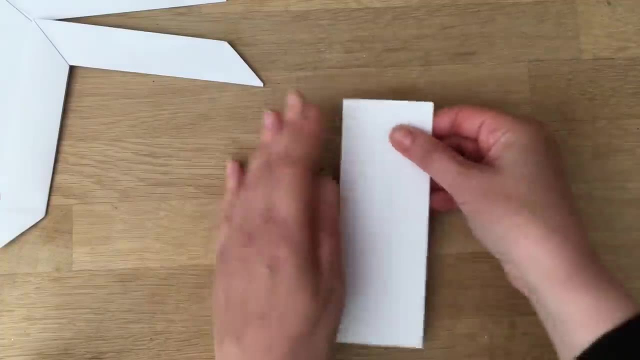 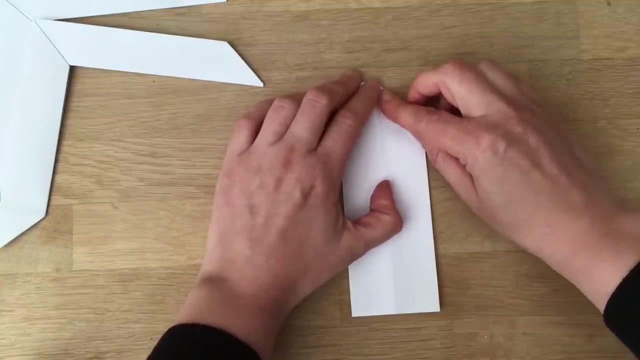 Again, make sure everything is lined up And then bring this over, Use your nail to crease it like so Okay, now I need to create a little triangle on this corner, Bring it up to the line. this time, Again, you do it with your fingernail. 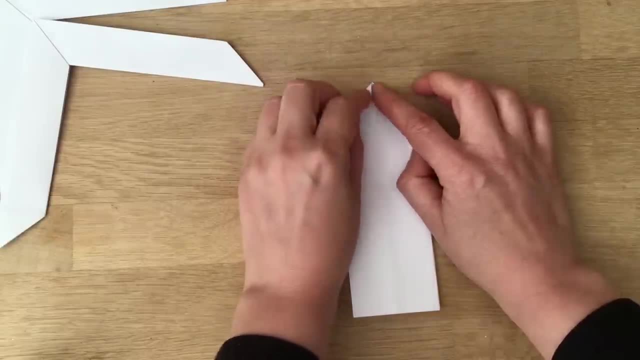 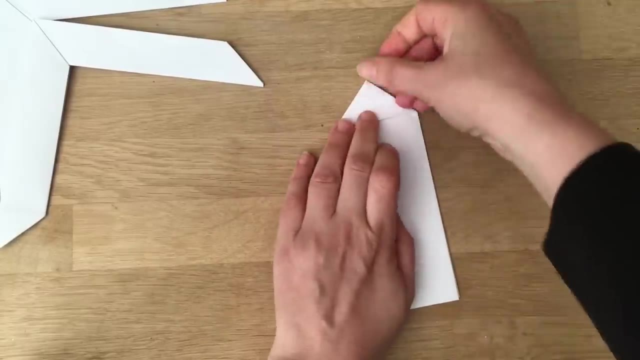 And bring this one out. If this is going too quickly for you, Just pause the video as you go along, okay? I think that makes the most sense, Because obviously I don't know what rate people are working at And you might all be working at different speeds. 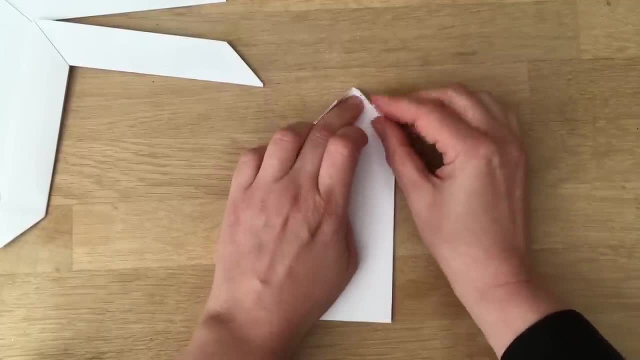 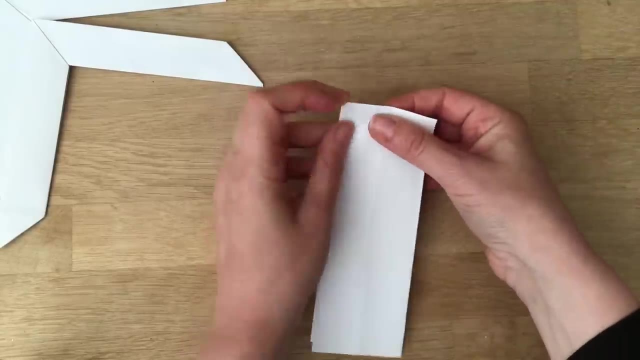 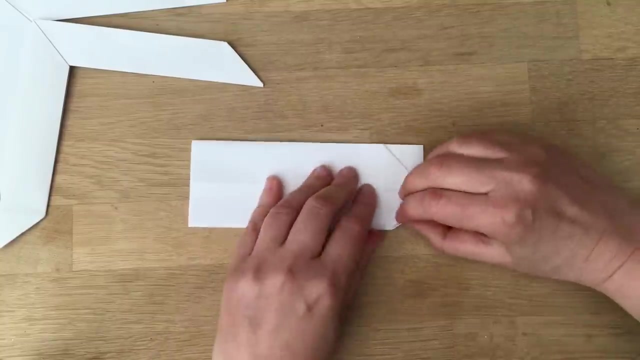 So bring that as neatly as possible. As neatly as possible, There we go, And I'm going to fold it in the other direction as well, because I will need a neat flap. There we go, All ready, There we go. Nice and neat creases. 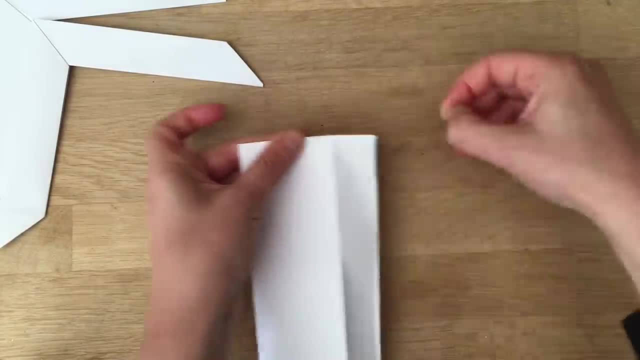 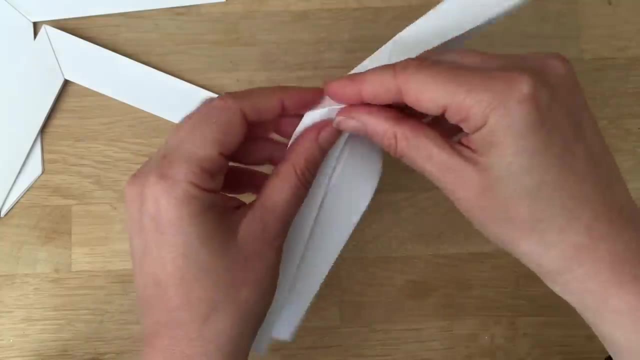 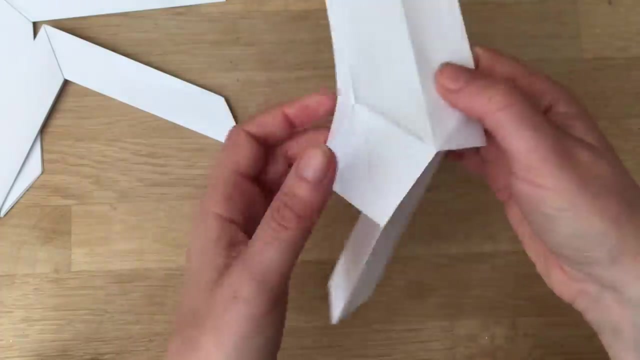 Okay, now I want to just emphasize this crease. I want to emphasize this crease because it's going to make things easier. And this one, And this one, And this one, There we go, And then I'm now going to bring this flap down. 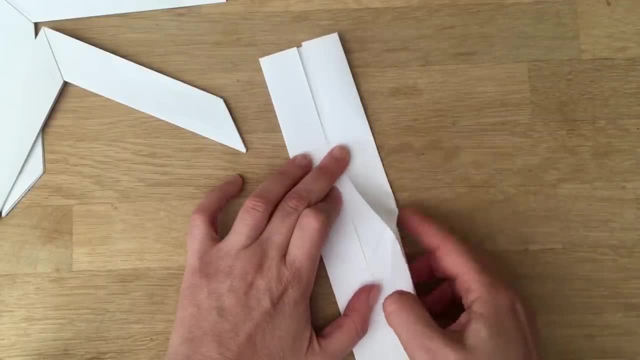 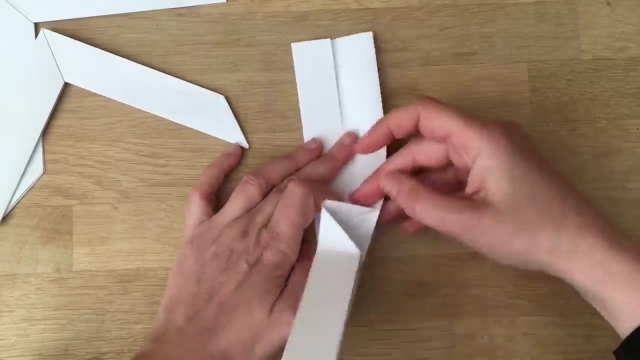 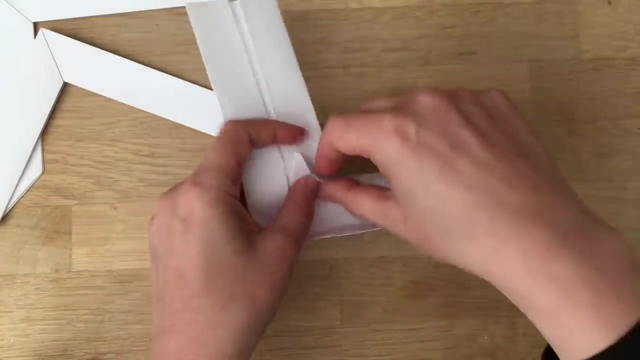 And as I do it, I'm going to give this a little tap And kind of push it in Like so To create like an inward pointing triangle, yeah, And also I'm going to put it flat against this back sheet. So this is flat now. 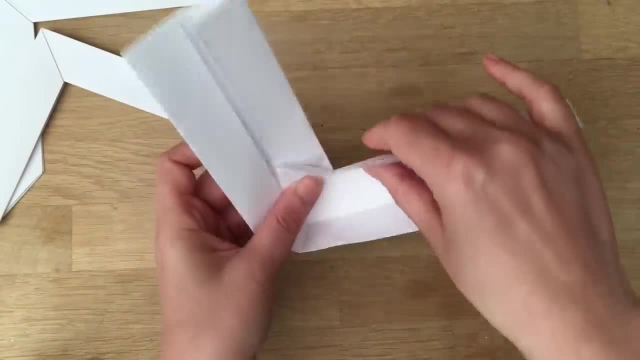 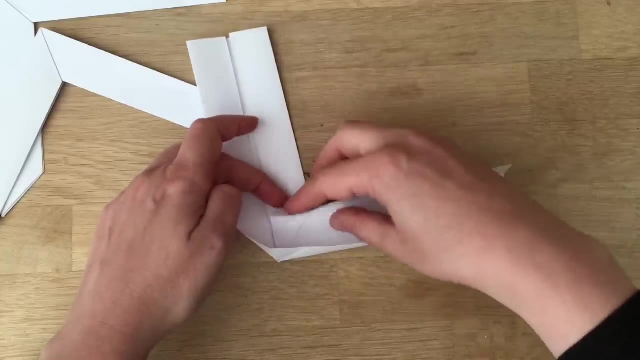 Okay, Like that, Now I'm going to bring this one down And as I bring it down, This flap here- Look at that- Just flaps down. Like so Now I'm a bit concerned because, look, I haven't done it. super neat here. 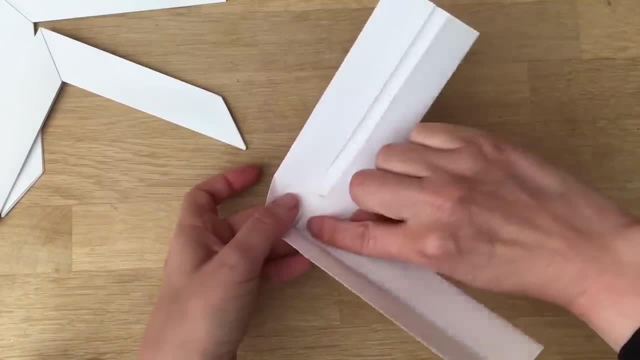 I'll keep going because it might still fly. But if this one doesn't fly as well, it'll be because I have obviously not aligned my edges properly. Naughty me, But let's keep going And see. So Now I need to bring the other edges down. 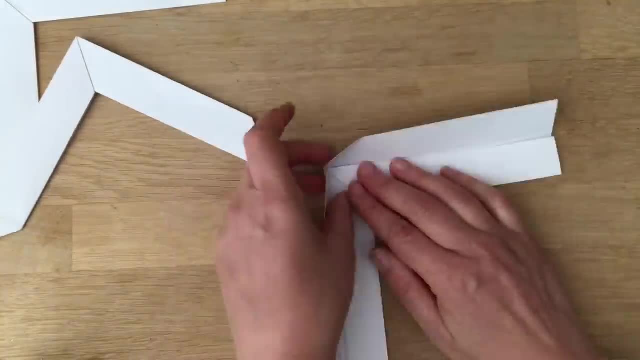 I'm going to tuck that in. Here you can see a little triangle forming, So I'm going to push that out, Like so, And you've got your basic flap, And then I'm going to fold it in, And then I'm going to fold it in. 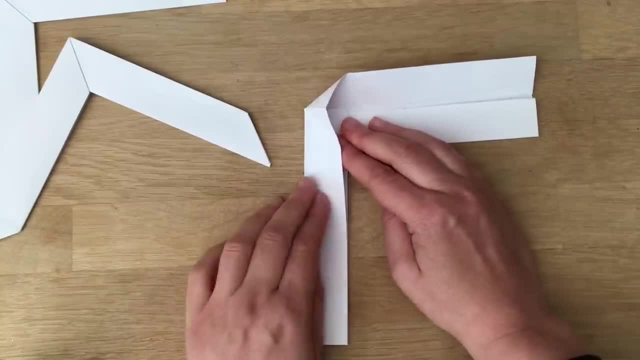 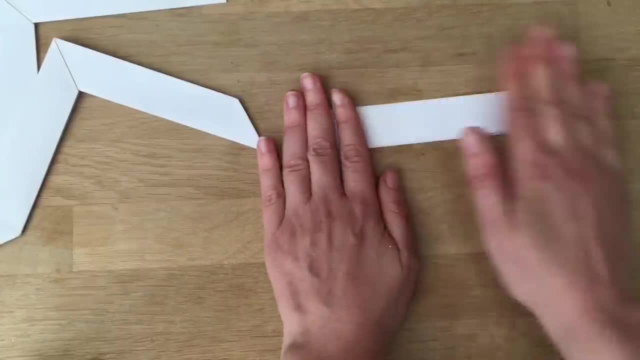 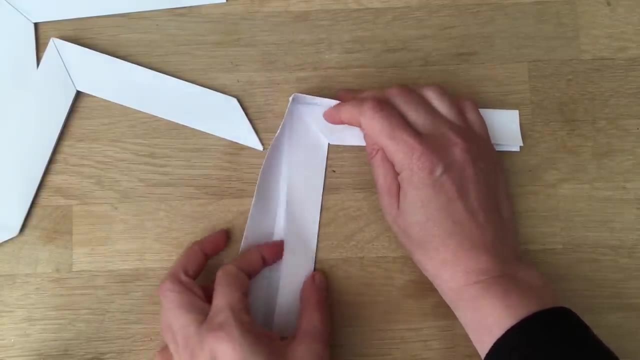 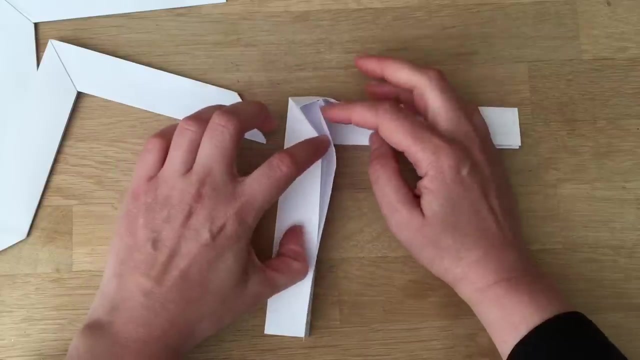 You've got your basic boomerang almost there, But not quite, Because I need to tuck things in so it doesn't fall apart mid-flight. So I'm going to open it again, Lift the inside, Push this flap under And then put my little pointy bit in the little triangle. 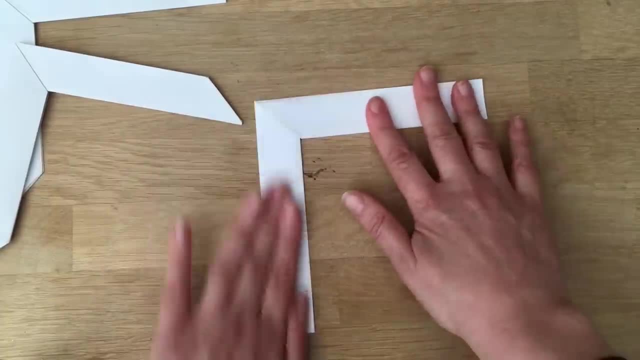 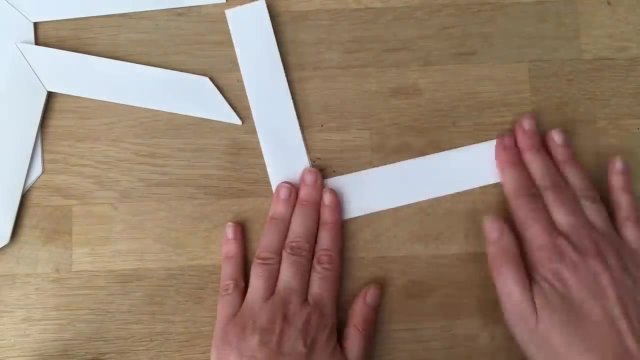 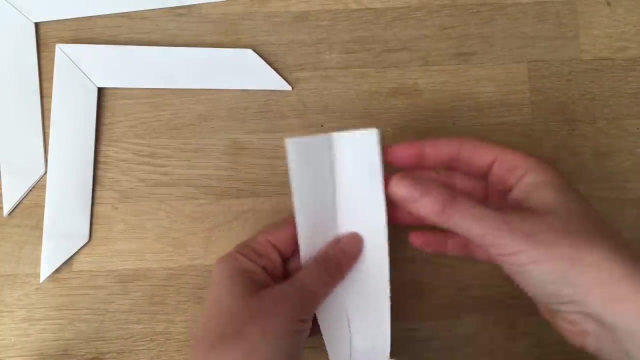 And this on the outside, like. so now it's all tucked in again. you can see I haven't been aligning my pages properly, have I? so, like I say, don't do as I do. I've done them super neat here. so these work, so we're fine. but this is how the boomerang is folded, just remember super. 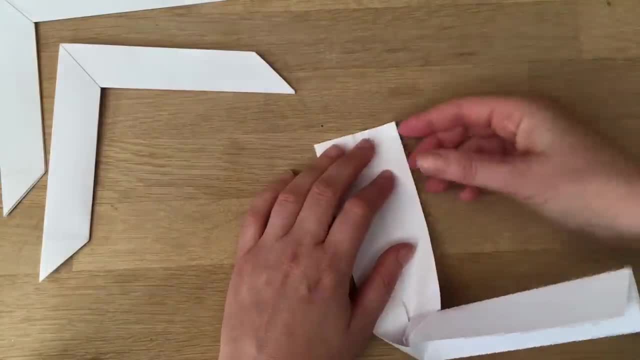 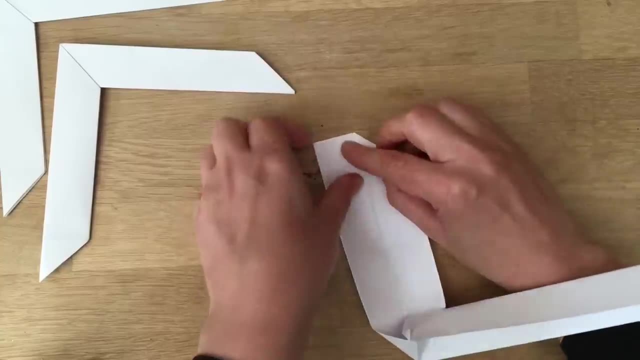 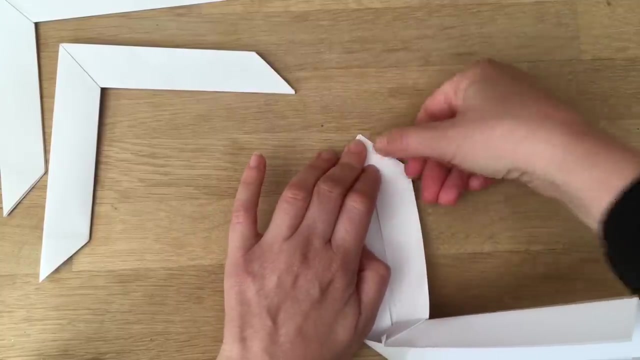 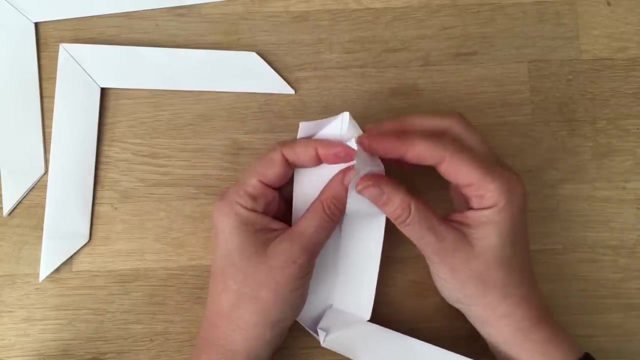 neat. so now we just need to do these little edges. you create a triangle at the top and then the same on this side, so and like, so, open them up. on this one I can tuck this in. so if it make it into an inside triangle, and then when you fold it, it means oopsies, it's coming. 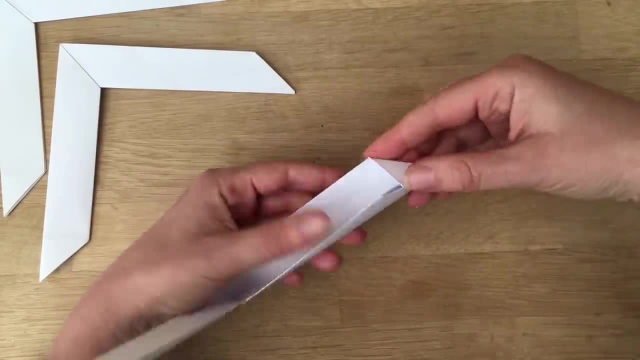 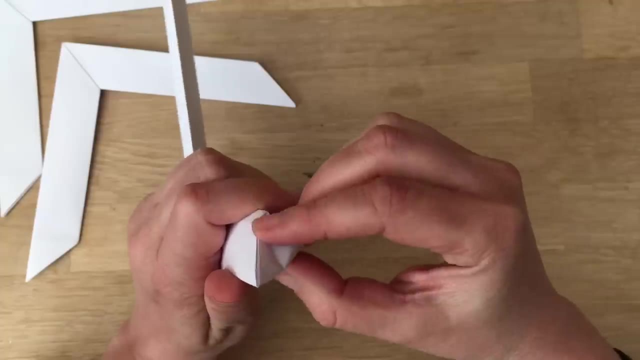 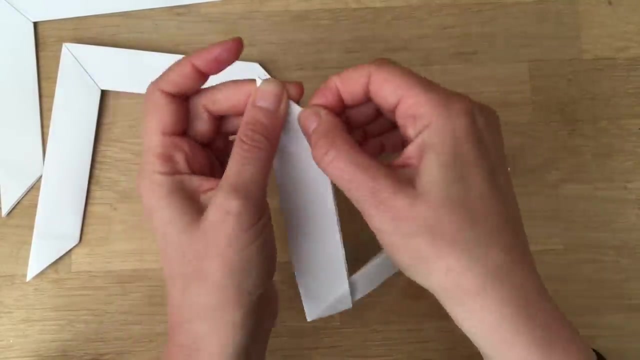 apart. then when you fold it, it means you can tuck this one in which also gives the boomerang. you know that extra stability in that it doesn't, it won't come apart. so tuck it in gently and as neat as possible. here we go. did you see? I tucked it in. 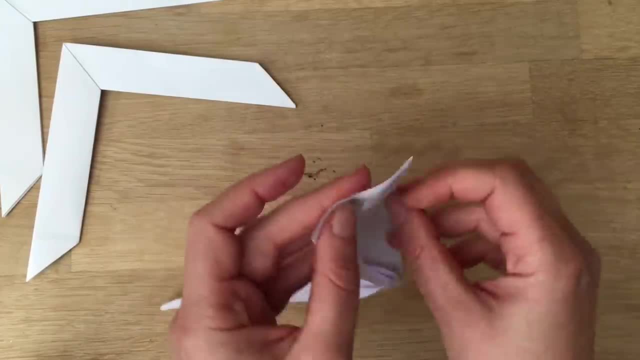 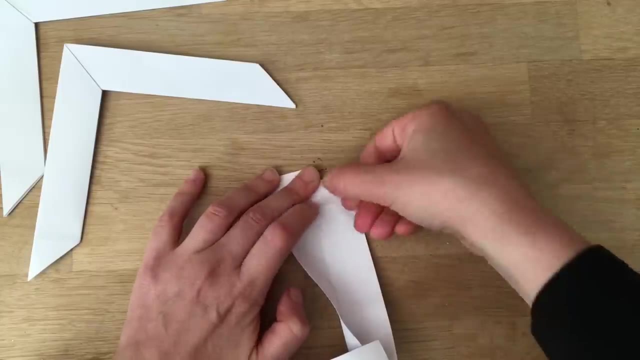 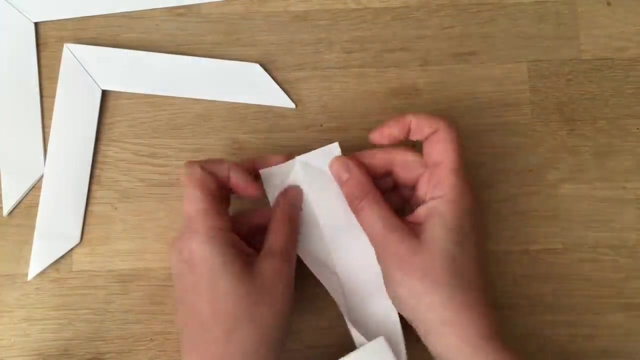 I'm gonna repeat the same on this side. but on this side you've got one sheet of paper and three on this side, so that's fine. but you carefully fold over the three, give it a good, and then you carefully fold over the one. you take open up the three, put it together and then you fold it over the three and you 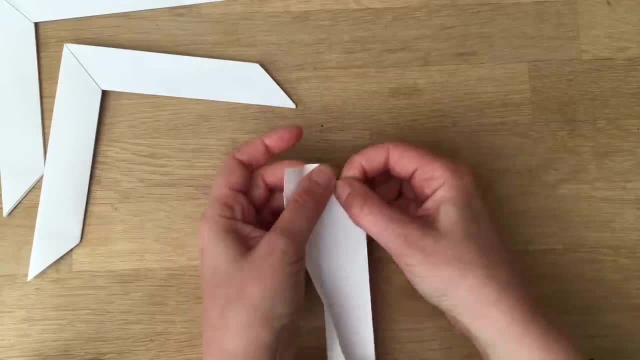 you fold it over the first one and you take open up the three and you fold over the three and you fold over the first one and you fold over the second one and you push it in, make a reverse triangle, close it and then you tuck the individual one in. 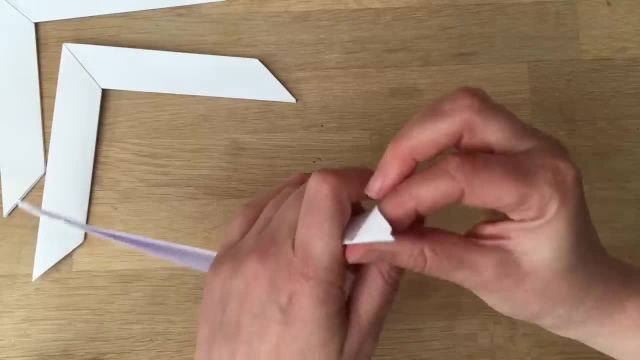 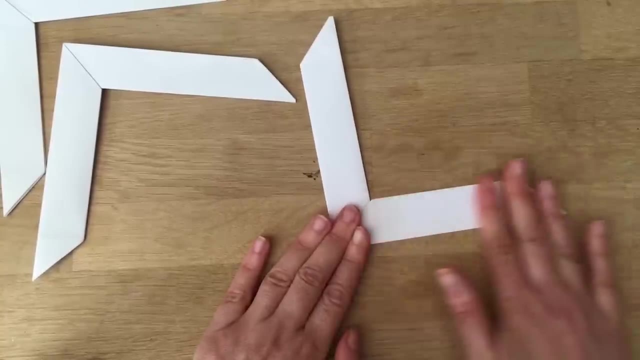 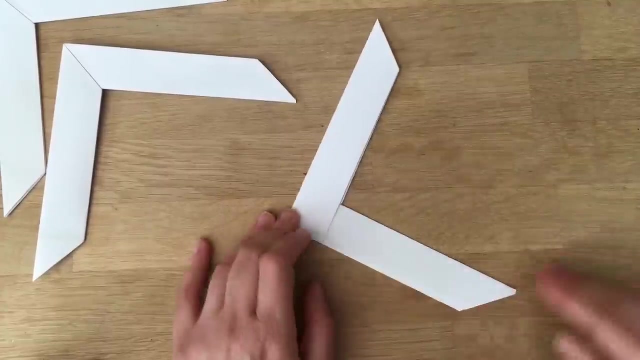 Now I'll be curious to see how well this one flies, as it's not my neatest. We'll see. Here we go. So now, before you get to fly, make sure everything is super flat and super straight and super neat. Now, when you're flying them, you will have to hold them like this: 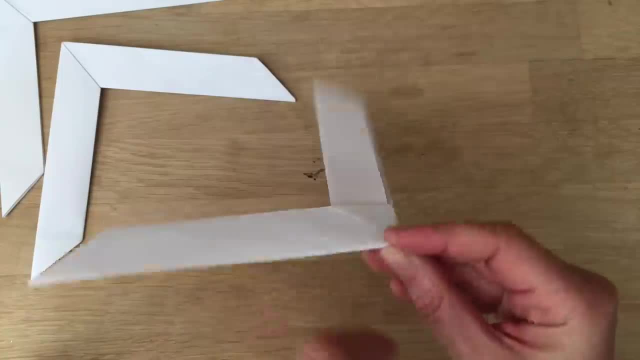 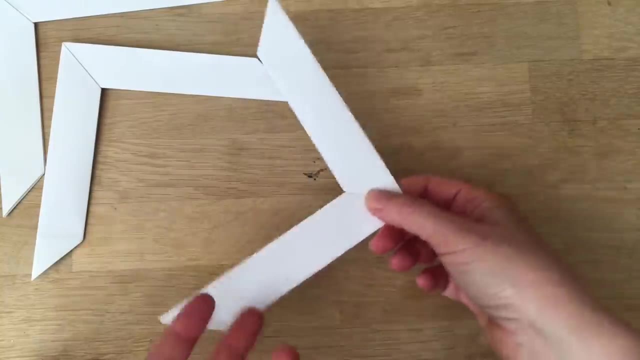 So you can see there's a line going diagonally here On this side. you've kind of got a square. You want this side to be up. This is for right-handed use. I'm sorry you'd probably have to somehow do this all in reverse for the left-handed ones, But you always have to hold it like. 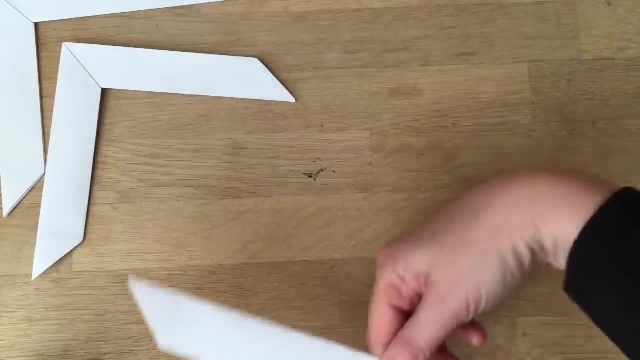 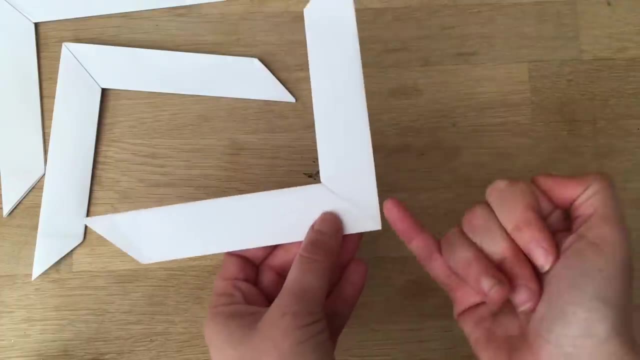 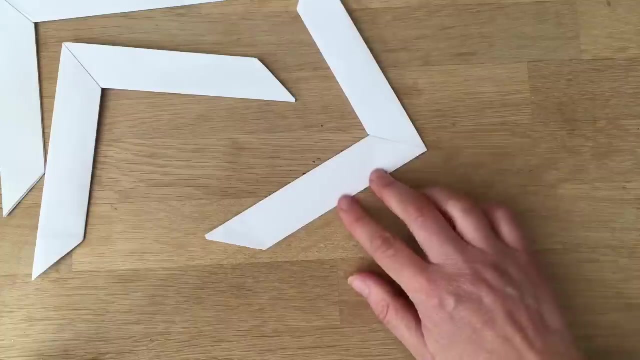 this and then you flick it like a frisbee. Now I know left-handed people who don't know how to use these and they do work for left-handed, But remember, this has to point up. So, yes, I'm going to go and get some help so I can film and flick at the same time and we can. 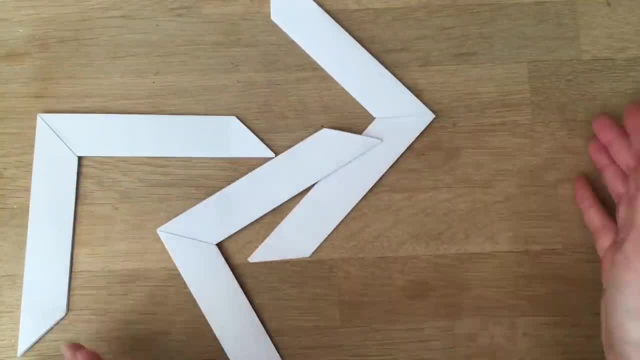 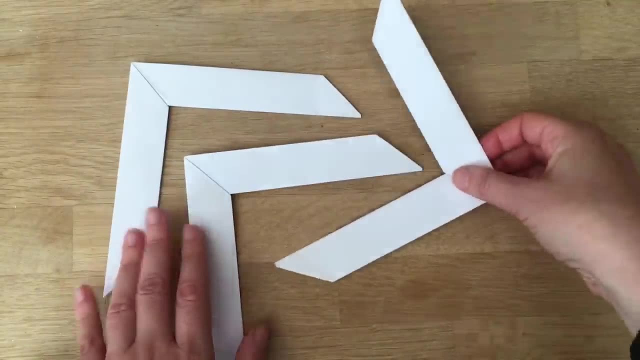 have a look at how well these work. Now, remember at this point it'd be really fun to decorate them. You know, use lots of colours, do them in black and white stripes, dots, whatever. Go and have a look at some Aboriginal artwork and maybe be inspired by the Aborigines and 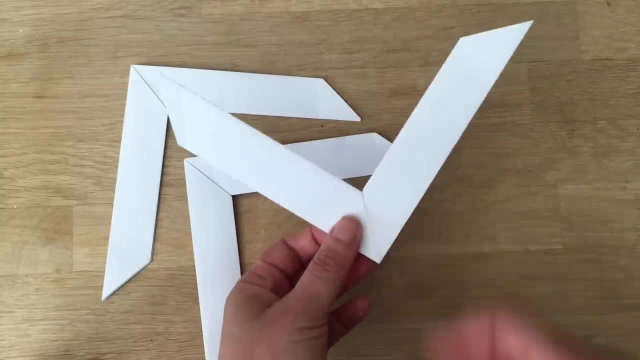 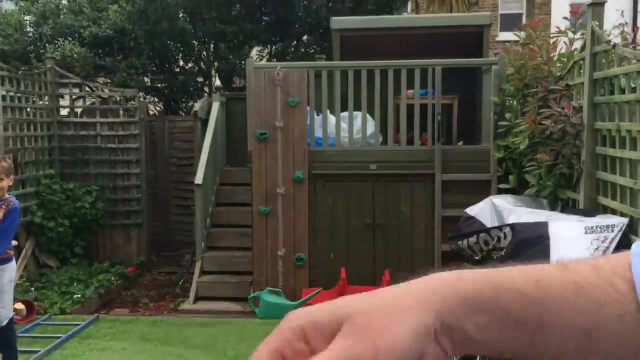 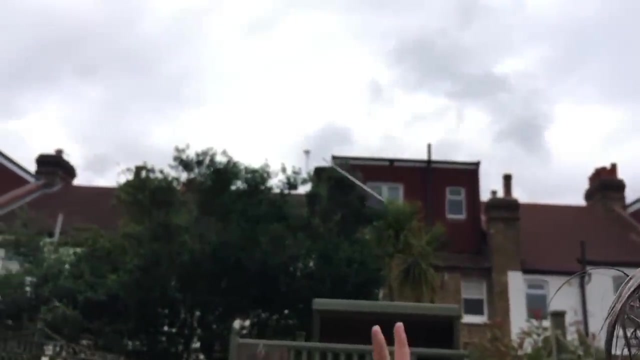 just make them your own. So anyway, let's go and see how well these work. So blink and you'll miss it. That came back so quickly. Let's have another go. Will he catch it? Oh, no, not quite. He's in slow motion coming back. We did miss it, though, as in 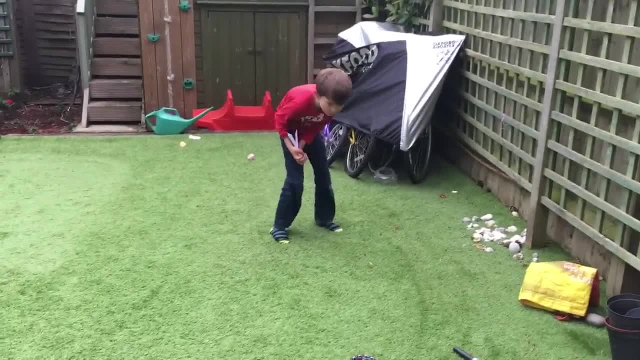 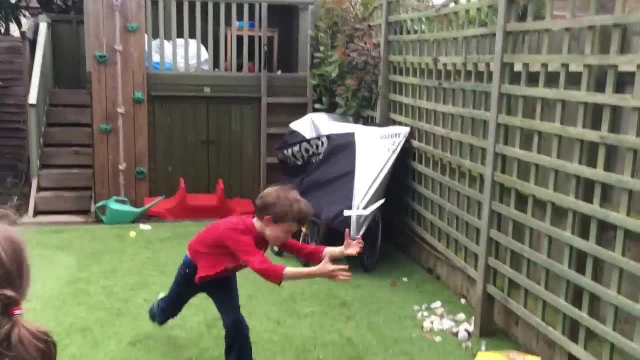 we didn't catch it, But it is coming back Now. the kids are having a go. Whoa well done. Let's see if we can do it again. Is it going to go? And oh, missed it. So let's see the. 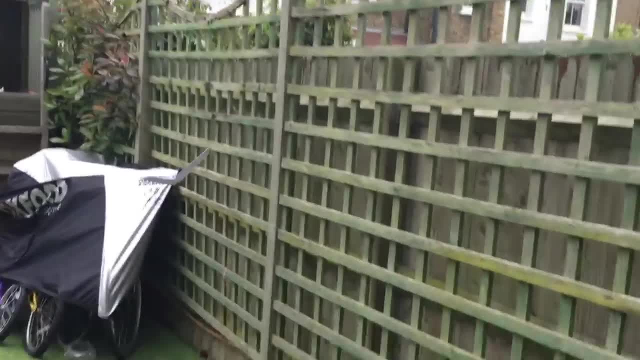 other one in slow motion. Let's see, There we go. Oh no, not quite So blink and you'll miss it. That came back so quickly. Let's have another go. There it goes, coming back. Woohoo, we've caught them. I just find these paper. 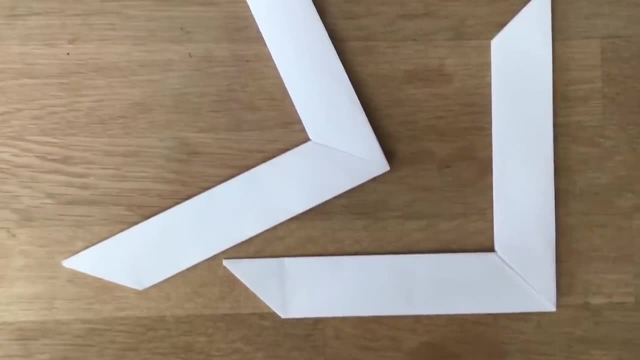 origami boomerangs: amazing, So simple and work really well. Now don't forget to subscribe to Redhead Art and see you here again soon. Bye.